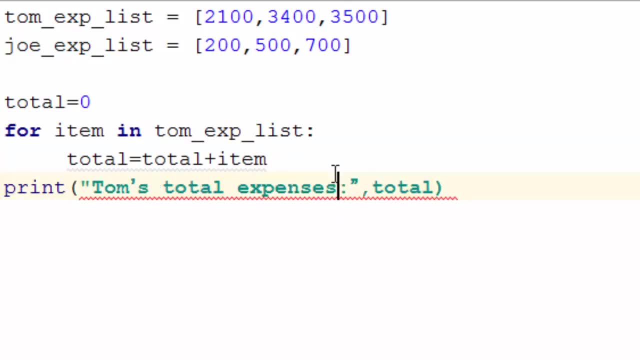 items And in the end you will print a total. I'm just copying and pasting the code from a different document just to save time on recording. So here, what you just did is you went over each of the items from Tom's expense lists and you added it to this variable. Now to find the 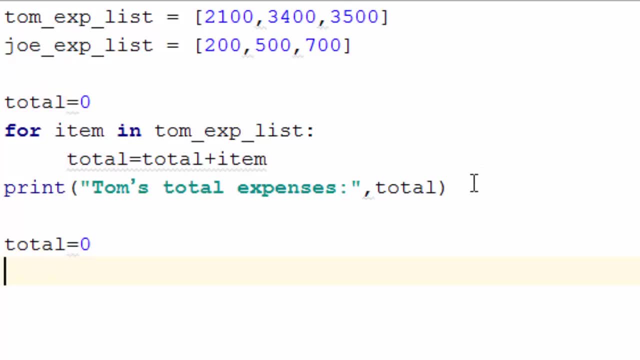 total of Joe's expense lists. you will do the same thing, So I'll just copy paste this code and I will replace this dádleIĞĞĞĝĞĞÉÆ guy with Joe's expense list, because the second thing you are doing is printing the list of total. 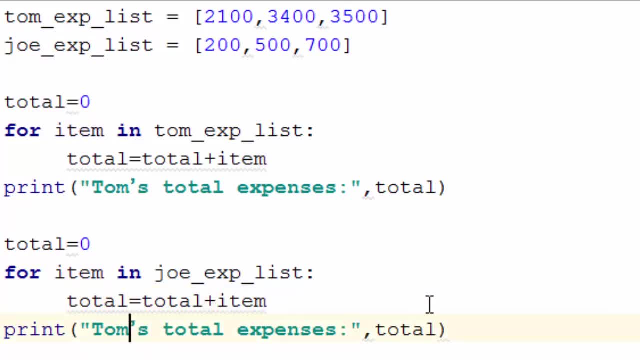 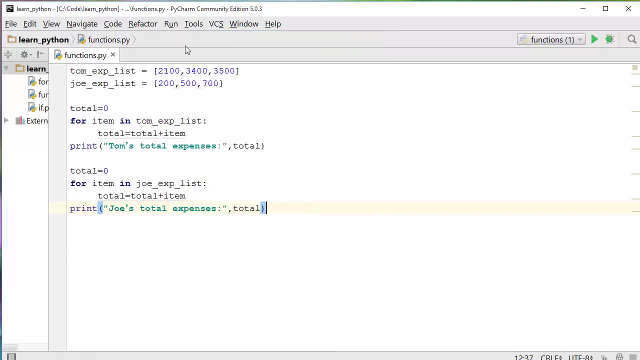 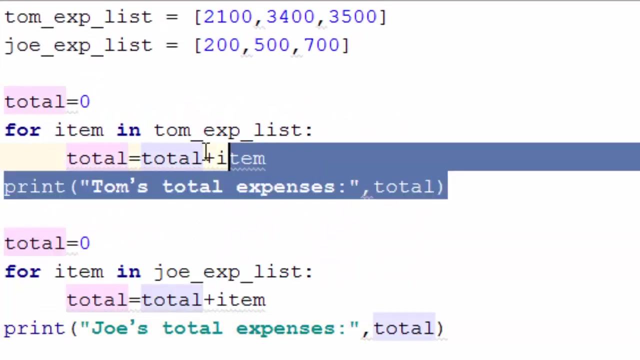 expense of Joe's list and you will say: these are total expenses incurred by Joe. okay, let's run the program. excellent. so when you run it, you got the total expenses from for both the people. the problem with this code is that you are repeating these three lines of code at two places. imagine: 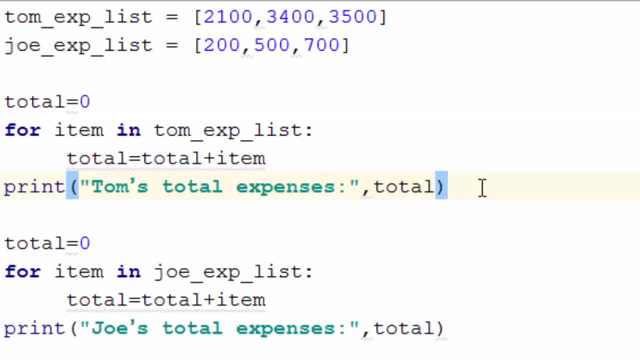 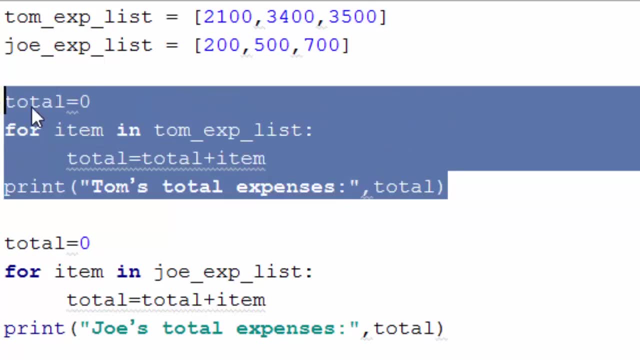 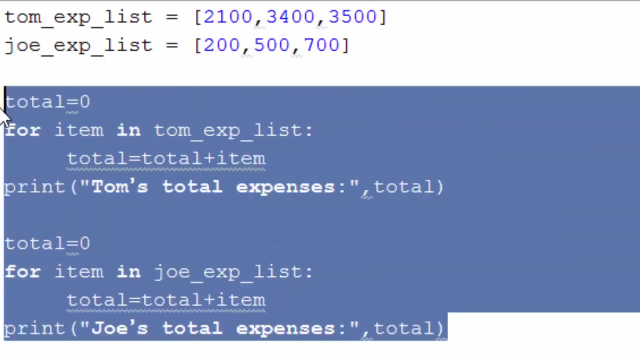 if you had 100 such lists, you will have to repeat these three lines hundred times, and that's very cumbersome. we can encapsulate this particular code into a function, so now let me write the same code using a function. so I'm going to remove this thing here. we will still keep our list. 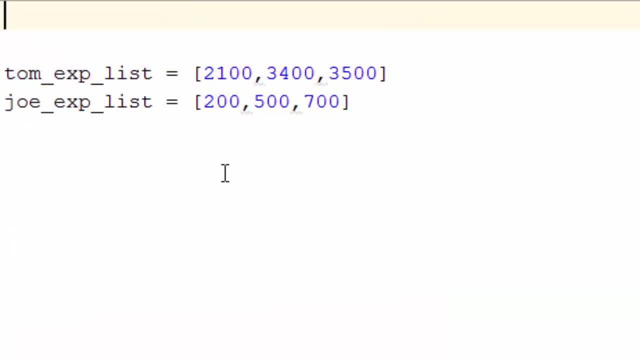 and I will start writing a function. so the way you write the function is: first you type def. def is a special keyword that tells python that I'm going to write a function. so calculate. total is the function name and exp is input. here you will create local variable called total and 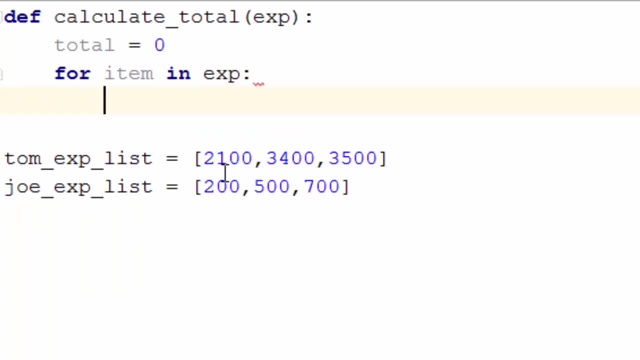 you will iterate through the items in exp and, by the way, these lists we are. when we call this function we are going to pass these two lists as an input. so exp variable will have a list. here you will say total equal to total plus item. in the end you return a total. 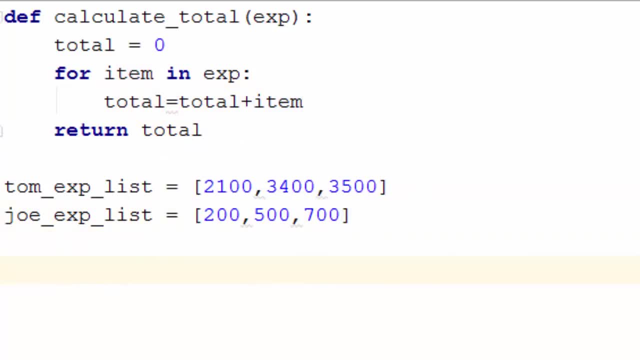 okay, the way you call this function is: you create another variable, Tom's total, and you call this function with Tom's list as an input. then, for Joe's total, you create one more variable called Joe's total and you again call this function calculate total, and you pass Joe's expense list as an input. now 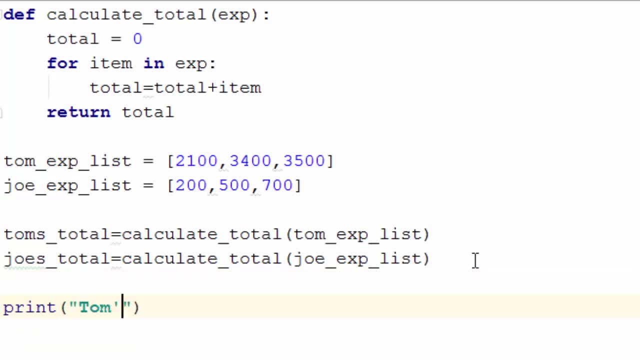 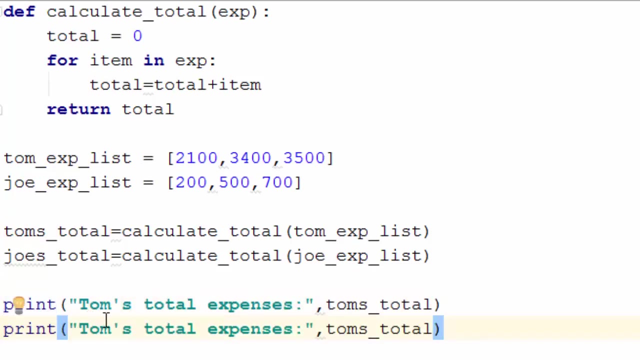 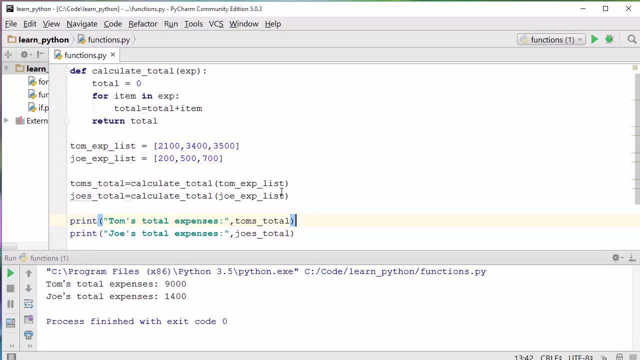 it's the time to print the total. so Tom's total expenses is Tom's total and I can just copy paste this code and I can say Joe's total expenses is Joe's total. okay, let me run it and see what happens. excellent, I got the same result. okay, now let me explain the way this worked is when you call. 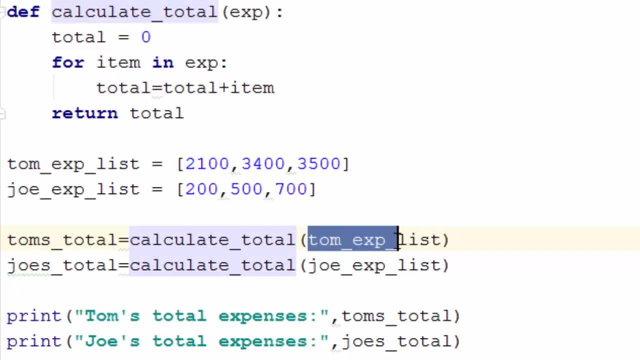 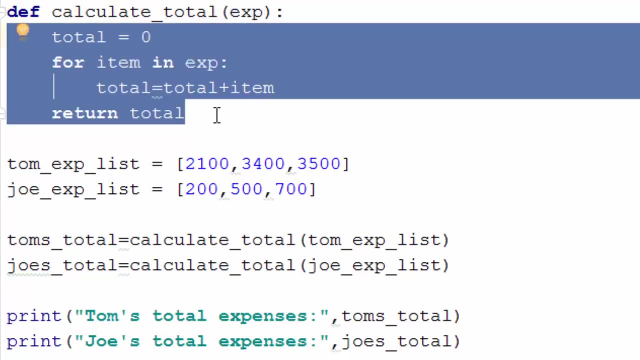 calculate total here by passing this list as an input. what happens is this list gets passed over into exp. exp is a local variable for this function. okay, and this much is a function body and the body of the function is defined by this indentation. you see this extra. 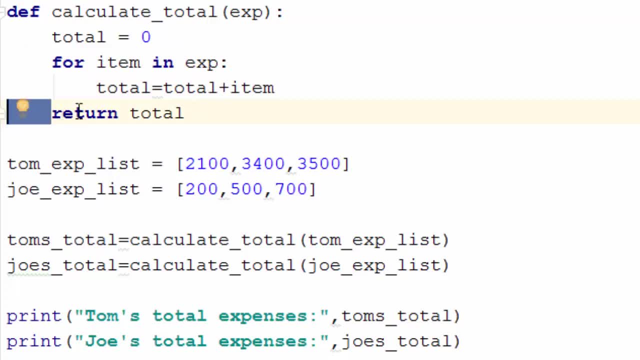 tag here. so whenever that ends, or whenever you return, the function body will end here. you will perform some operations, you will create a local variable, you will write it to the items and in the end you will return. so this thing, total, here is called a return value, and you return a value from a function by using 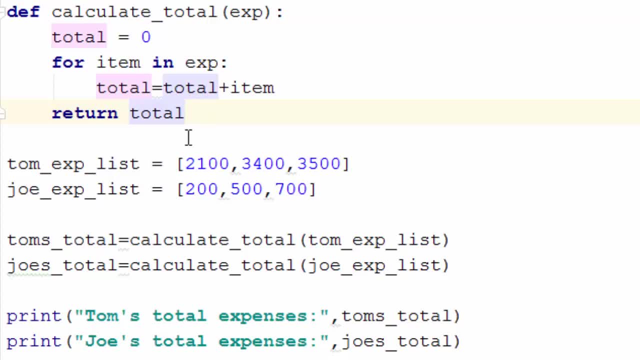 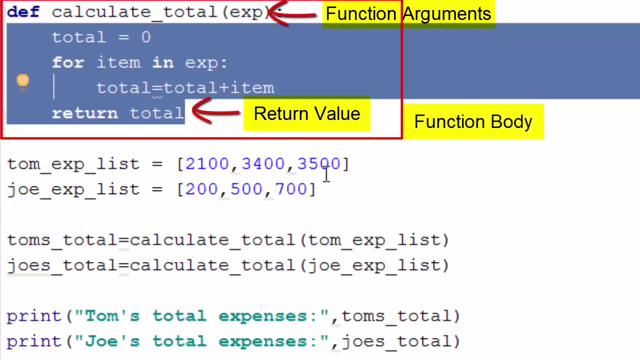 using this return keyword. okay, so these are the basic components to remember. so number one is a function argument, number two is a function return value and this whole thing is called function. okay, so if you compare with this again with a dishwasher example- just imagine this is a dishwasher- then this is an input to 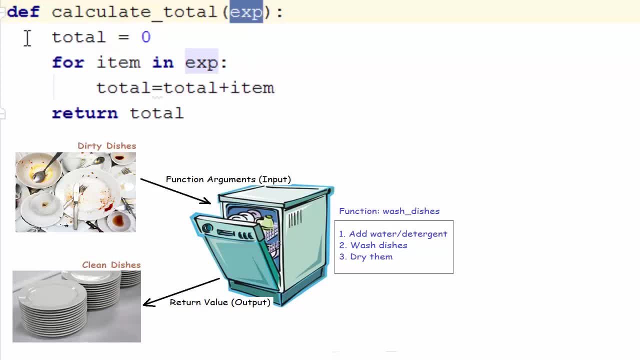 the dishwasher, which is your dirty dishes, and these three lines is the set of steps that dishwasher is performing, like adding water and detergent, washing the dishes, drying them out, etc. in the end, this return statement returns you the clean dishes, which is an output. okay. so that was a quick comparison with a dishwasher. now let's work on another. 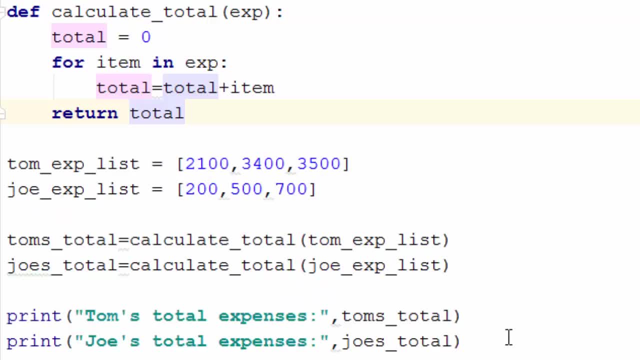 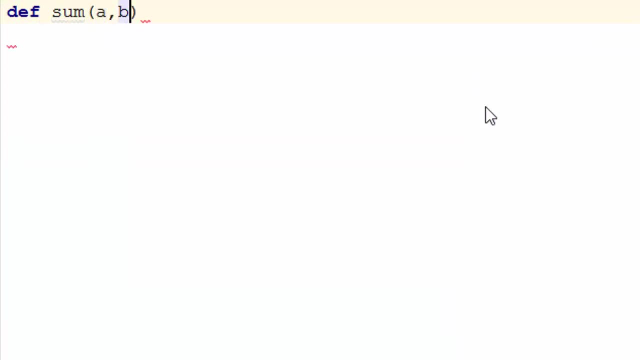 example, and this one is going to be very, very simple. let's say you want to do sum of two numbers. you can do it using a function. so I can write a function. let me erase this code. I can write one more function called sum and a comma B. so if a and B are the arguments to this, 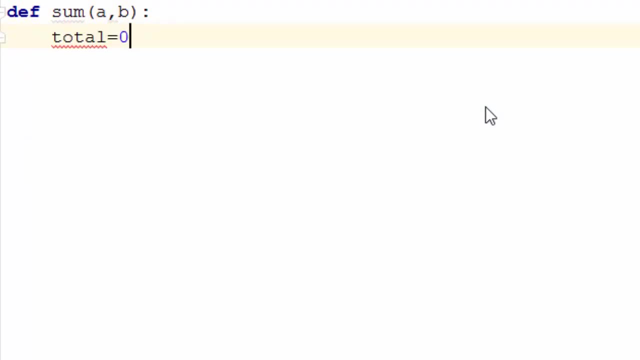 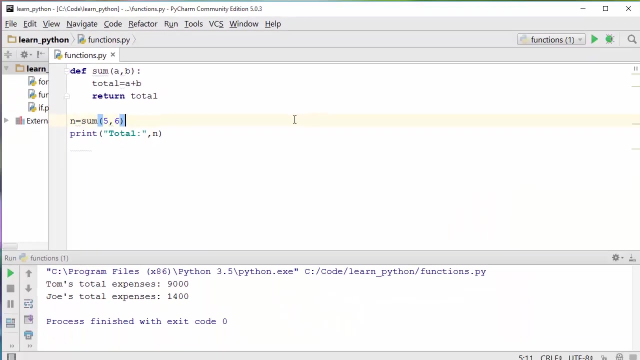 function. here you create a local variable, total equal to zero and or rather total equal to a plus B. you can just return it. return total, okay. and you can say: sum five and six. okay, now tell me what will be the output of this program. so when I run it, as you all expect, I'm going to get eleven, because five plus six is eleven. 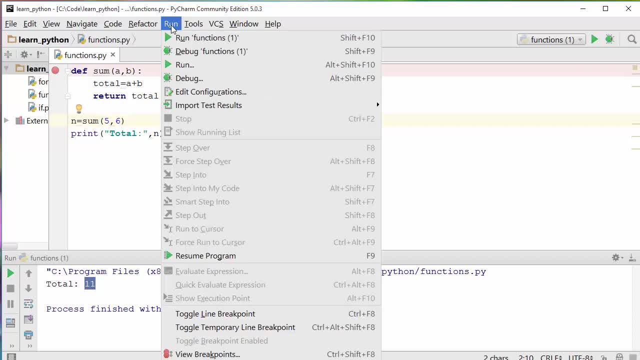 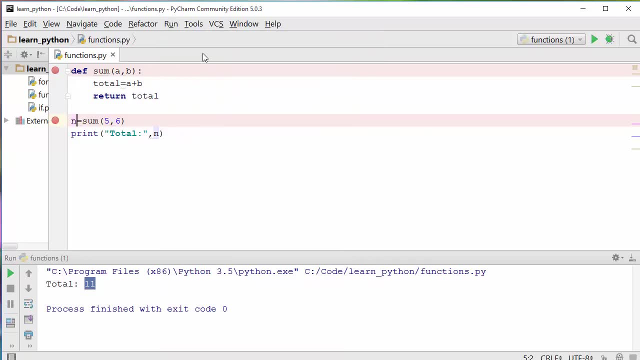 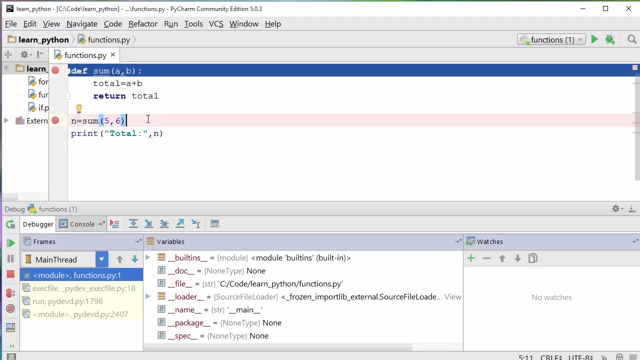 what happened here is: let me debug the program and then I'll explain how it worked. I will a breakpoint at do these two places. I will say debug okay and I will say okay next. so it first defined a function, it. we have not called the function yet. 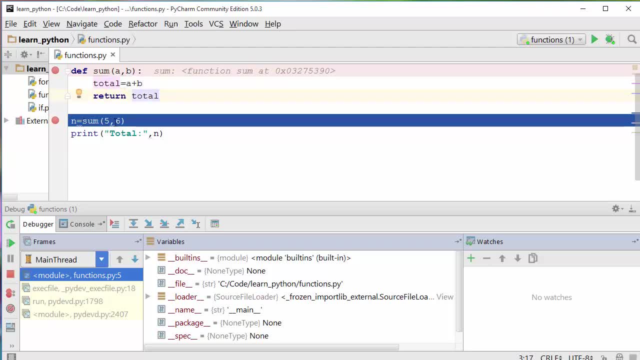 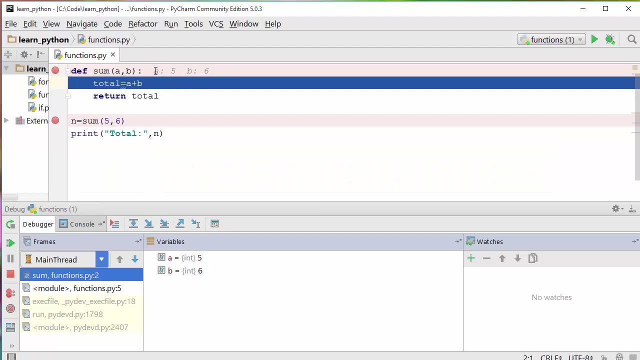 that's why it didn't go here. okay, we are calling function here. so when you say go inside the function, let me see which one this one is step into. so stab into next. as you see here, a has value phi and B has value 6, whatever you pass from here. 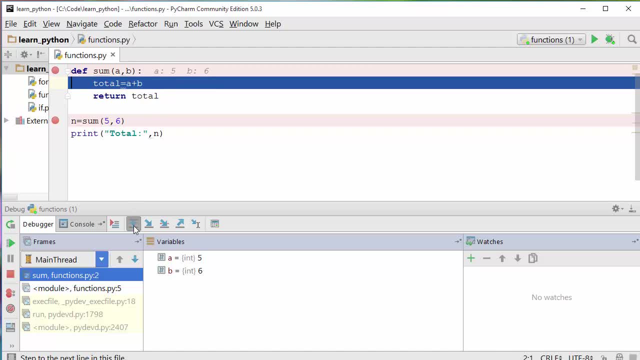 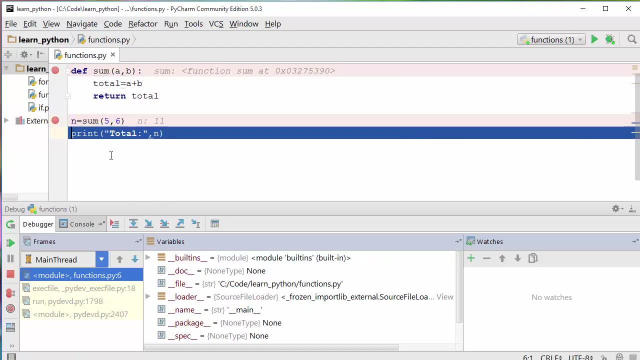 this guy will get those values. and when you say next, total is 11, and now we are returning this total, so this total will now get placed into this end variable. next, as you see, n still doesn't have any value. when you say next, at that time n gets 11.. 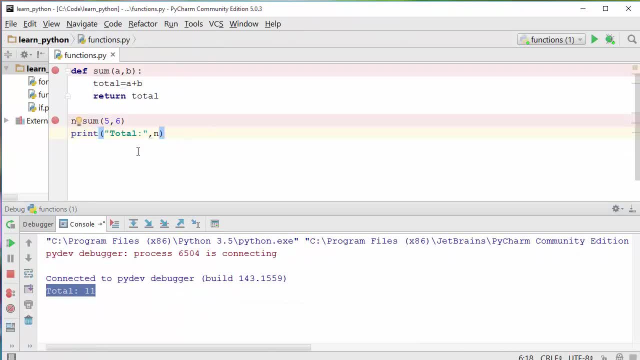 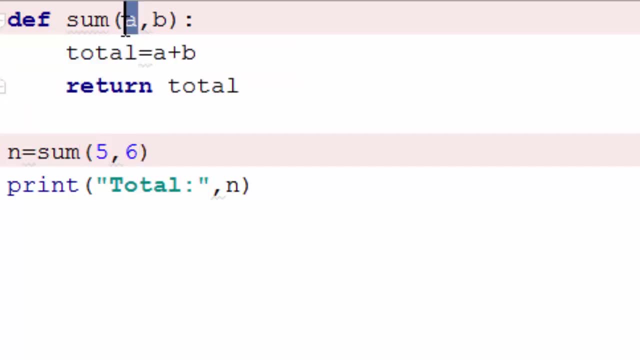 okay, if you check console, we got total 11.. now the way we are passing function arguments here is by order. so if you want to pass something in, a, you put that value here as a first value and b you put that as a second value. let me print those values here. i will say: 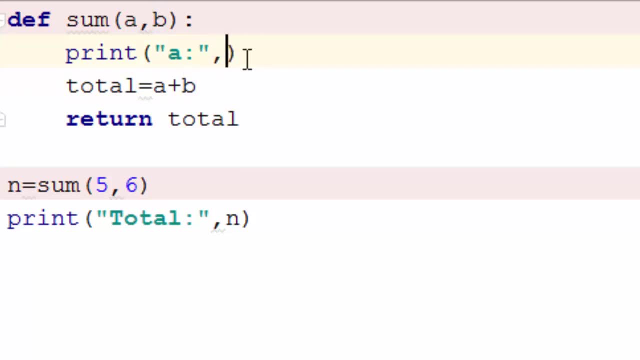 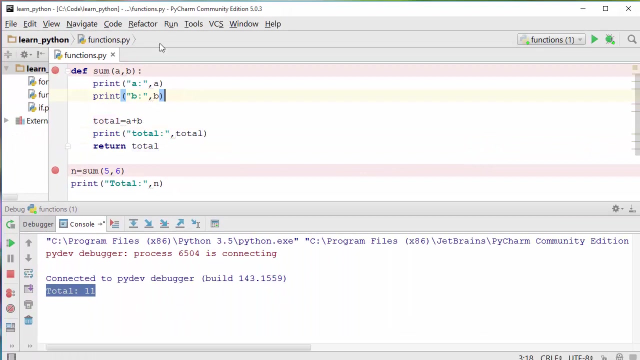 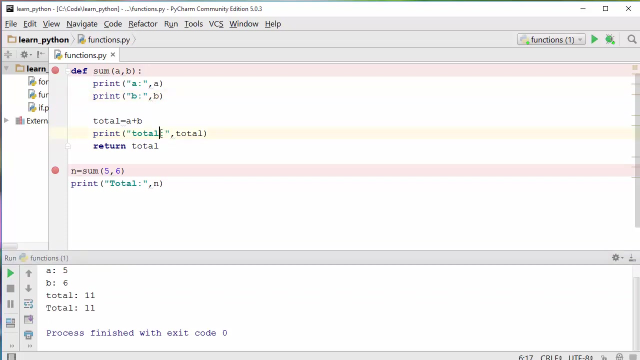 print a is a, then let me just copy this couple of time. b is my b and i will also print total before returning. so my total is total. okay, let me run it. so if i run, it is five is six, total is 11.. and total inside function: inside function: this is total. outside function, okay, 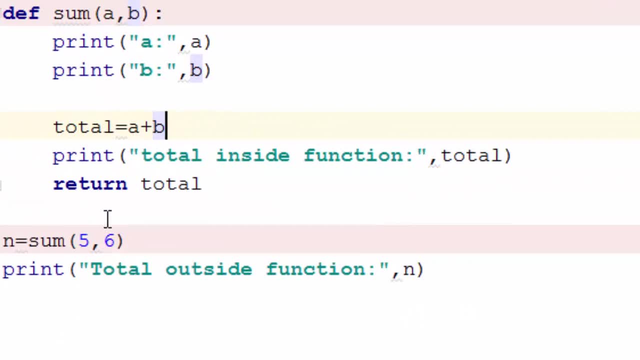 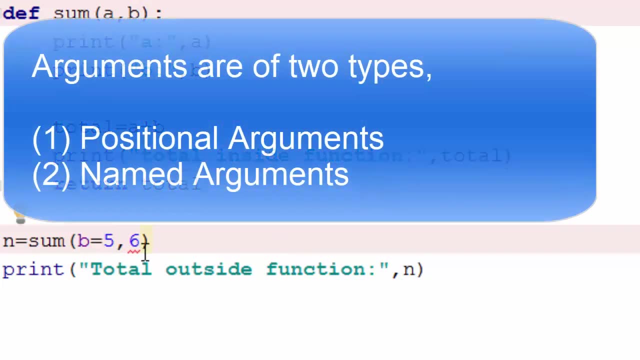 now what if i want to pass b first and then a a second, so you can use something called name argument. so if you say b explicitly, say b equal to 5 and a equal to 6. what's going to happen is then it will not go by order. these are called named arguments. 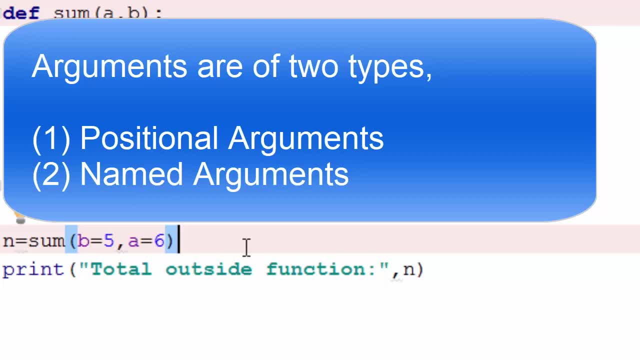 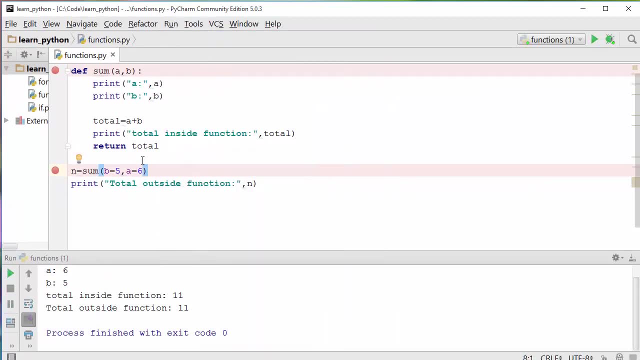 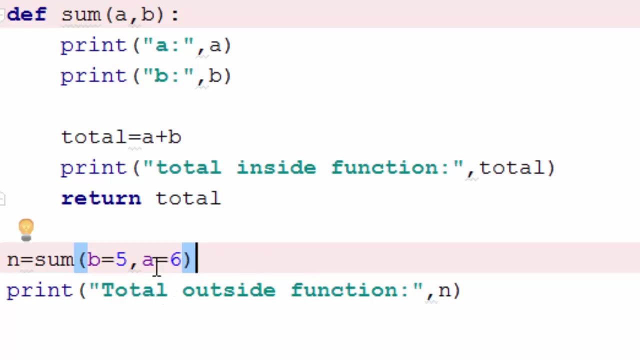 and the other ones were not. they're not named arguments. they were basically using the order. uh, let's run this voila. so a is 6, b is 5.. if you have a long list of arguments and you want to be specific about which argument has which, 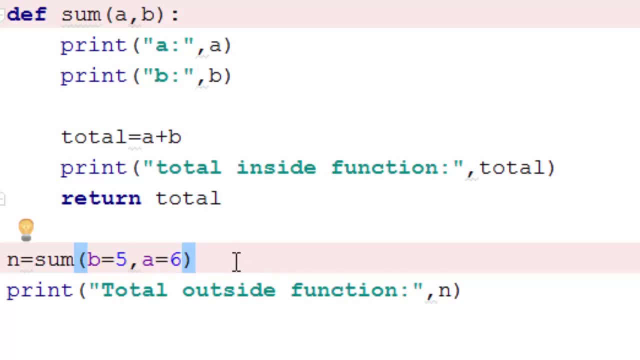 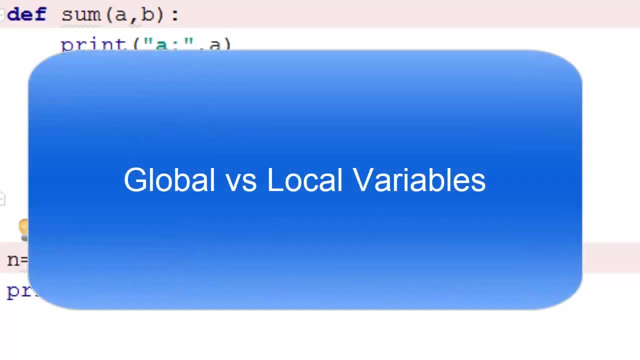 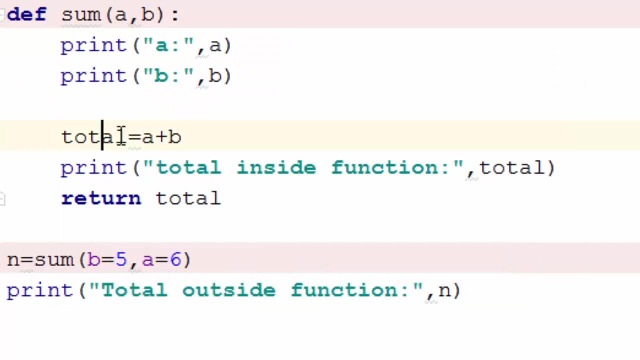 value, you can use these named arguments. otherwise you can just use plain order. cool. next item is global versus local variables. so until now, all these variables that we created here- a, b, total- these are local to this function. if you try to access these variable here, for example, let me print total. so we have defined total variable here and all i'm trying to do is 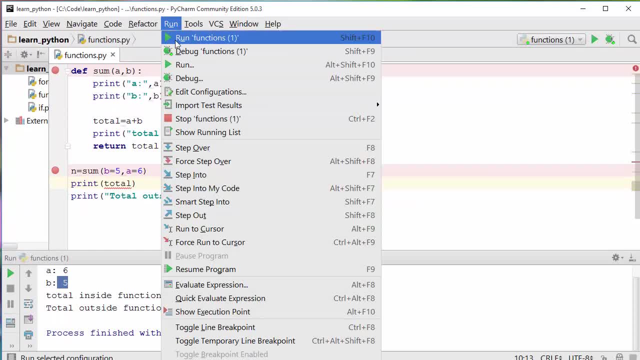 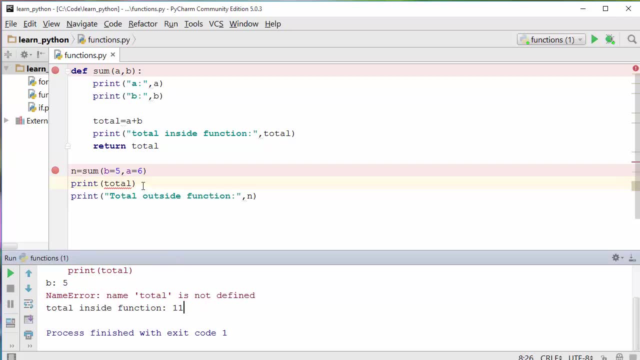 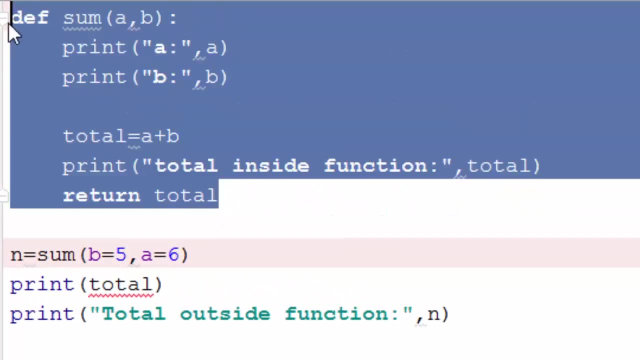 print total. but you see this red line. it says okay, let me run it. it says name error. name total is no, not defined, which means total is not visible outside the function body. total is only visible inside the function body and my function body is this much okay. so what happens if i have? 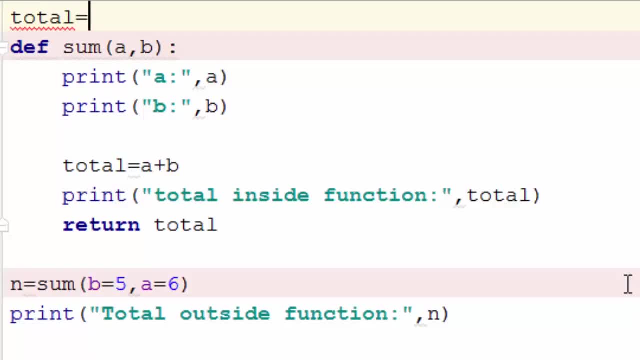 one more variable called total outside. so if i have total equal to zero and if i say total outside, the function is total, okay, let's see what happens. total was zero here and here we assign a plus b value. we are printing total inside the function and then outside the. 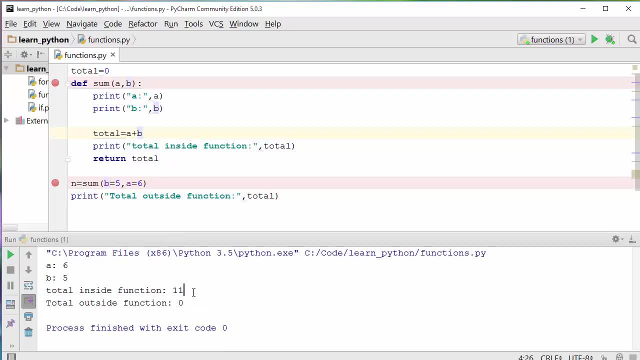 function. let's run it great. so total inside the function was 11, but outside it is zero. so you see, this variable and this variable, although their names are different, their names are same, their values are different because those variables essentially are different. this one is called a global variable because it is our. 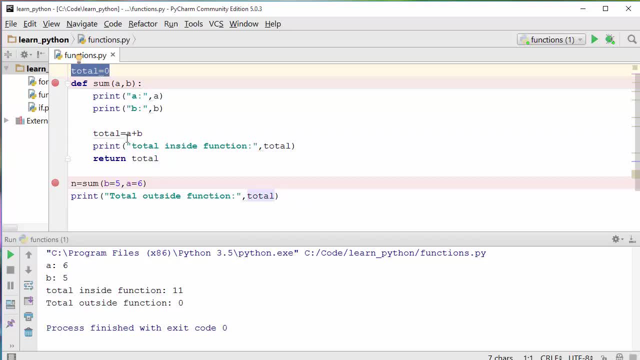 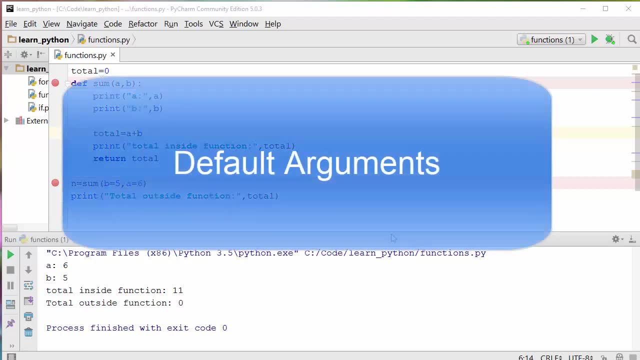 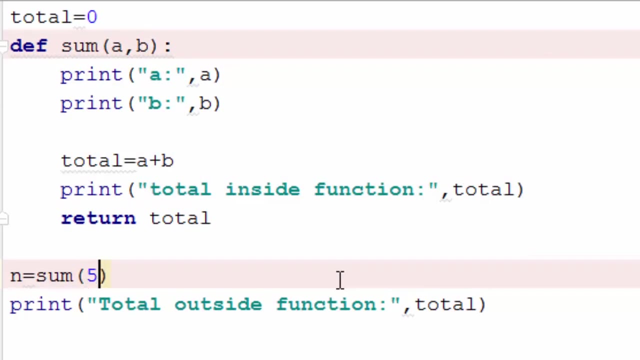 any function, it can be accessed anywhere. this one we created locally, so it is a local variable. okay, let's now talk about default arguments. I will just revert this back to what it was originally. here we are passing two arguments to the function. what if I don't want to pass the second argument, if you don't want to? 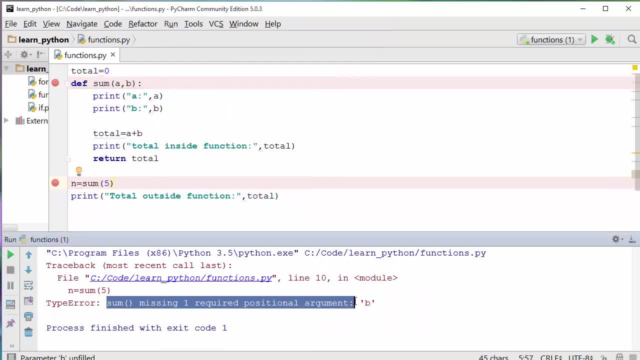 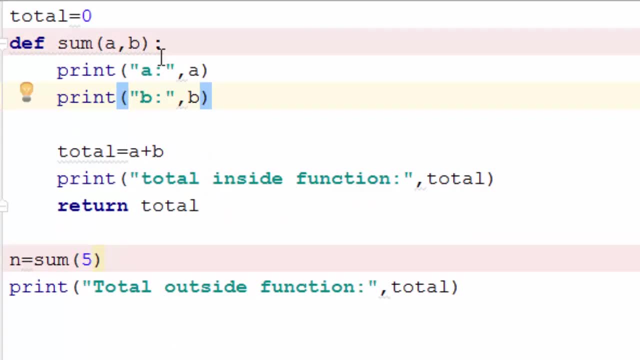 pass second argument and if you run the program it won't run because it will say it is missing the argument. okay, but sometimes you may have a default value for the second argument. so I'm making an assumption in my code that if my function caller doesn't pass me an argument, assume it to be zero. so when 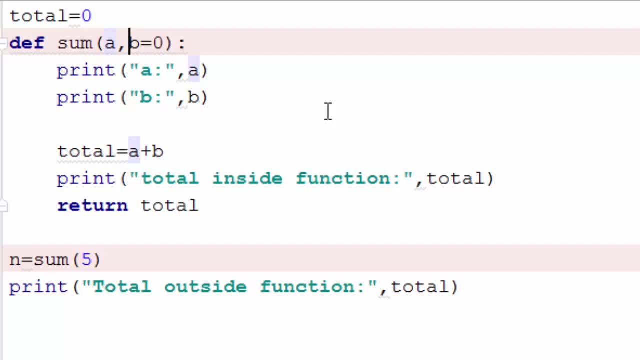 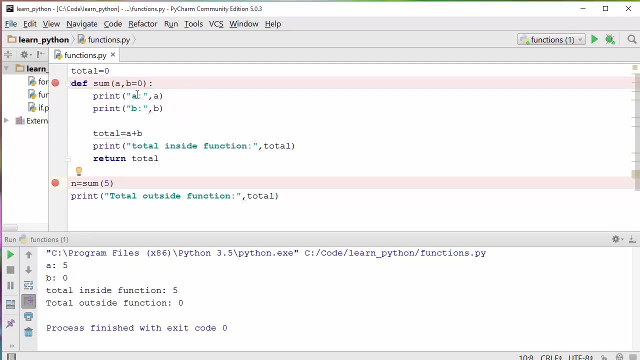 you say this inside of a function argument: when you assign a specific argument of value, that becomes a default argument and if you run the program, it won't run because it is default value for that argument. so now, if you run it, it will work fine. what this is saying is: if you don't pass me the second argument, then I am going to 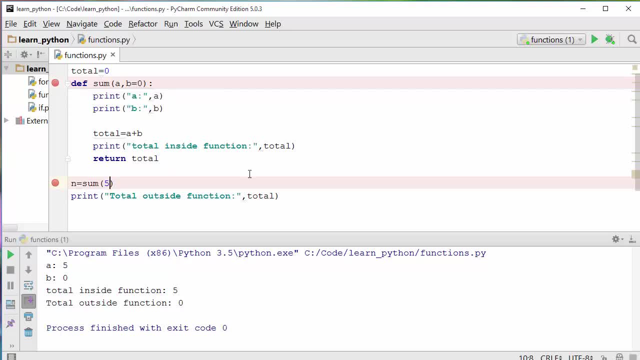 assume it to be zero. but hey, you are free to pass the second argument. if you pass this, imagine what's gonna happen. it's not gonna make that zero. let me run it and prove it. excellent, so you see, here B is 8 and this didn't have any. 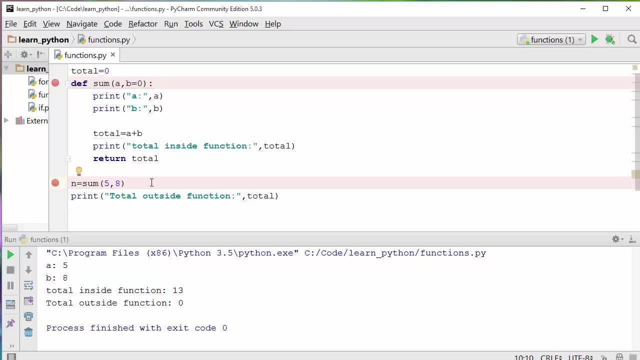 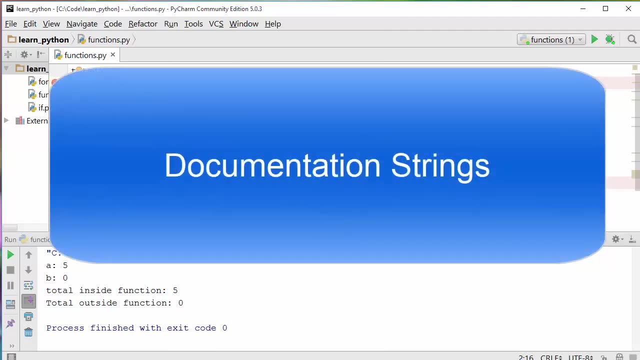 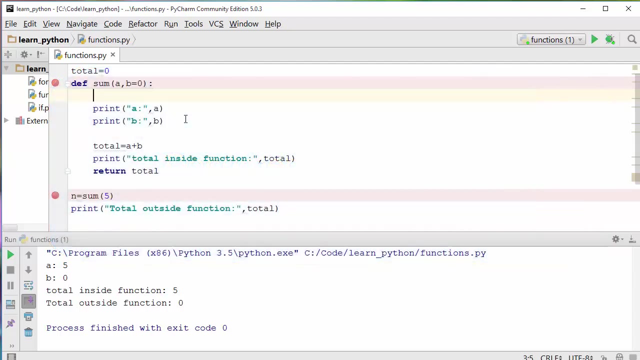 effect. so this will have any effect only if you don't pass the argument. okay, we want to conclude our session by covering document strings. real fast documenters and strings are nothing but a way to document your function. this function was very simple. it was just doing a sum of two numbers. but you might 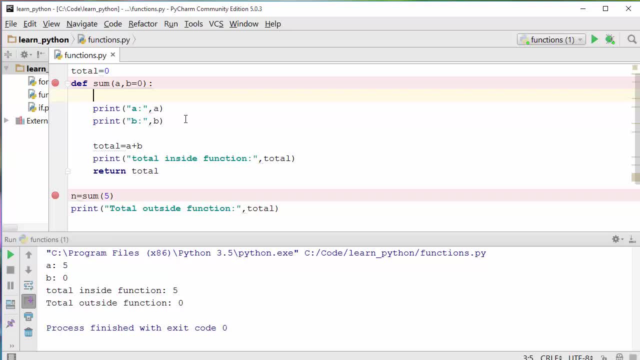 have a big, complicated function. in that case you want to write some documentation to explain the color of that function and you want to write some of that function on what that function is doing. what does it expect as an input and what does it expect as an output? so the way you write documenters and string. 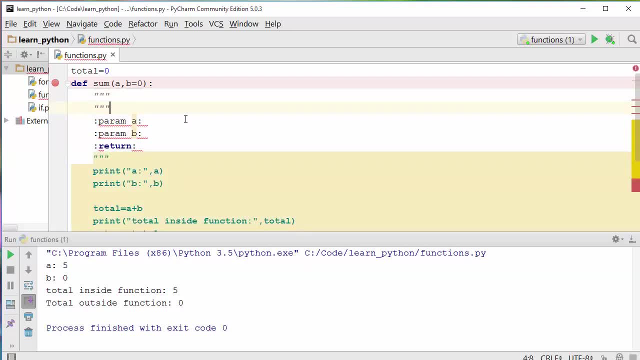 is you use triple quotes like this and by default, pycharm is giving these default documentation. but if you're not using pycharm, if you're using idle or something, you have to manually type all these things in. okay, so let me just remove these things and manually type it in, so this function. 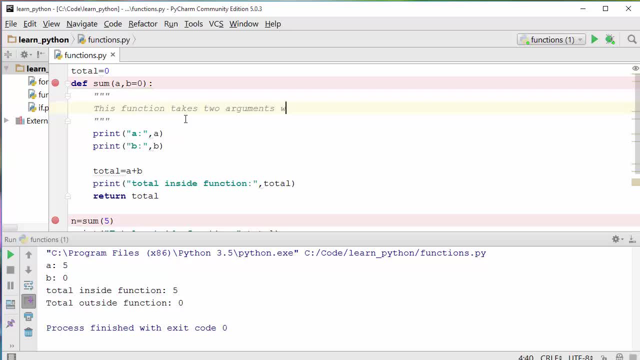 takes two arguments, which are integer numbers, and it will return sum of them as an output. so when you do this, if someone is calling your function, if he reads these lines here, he will get an idea on what this function is doing. so this is called a documentation strings. 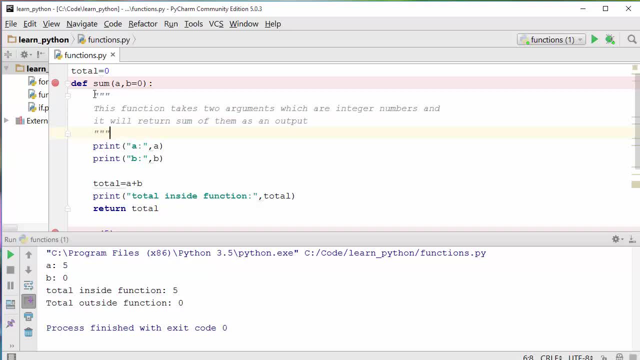 and it is a multi-line strings started and ended with triple quotes. all right, we cover pretty much everything about functions. uh, don't forget to work on these sample exercises. at the end of my every video, i give these sample exercises to for you to work upon, and these are extremely useful and it will help a lot in your learning. thank you.